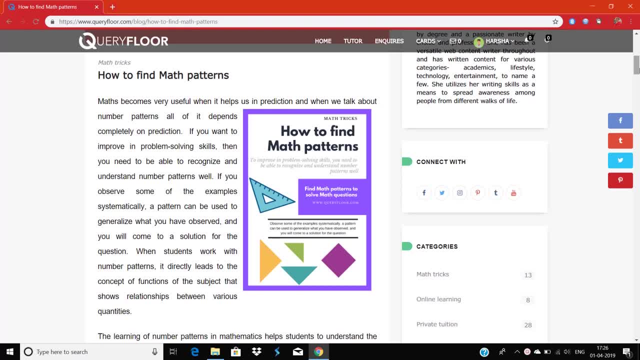 the numbers. If you observe some of the examples systematically, a pattern will come out. What you have observed and what will come to a solution will be of the same pattern. When students work with number patterns, it directly leads to the concept of functions of the subject. 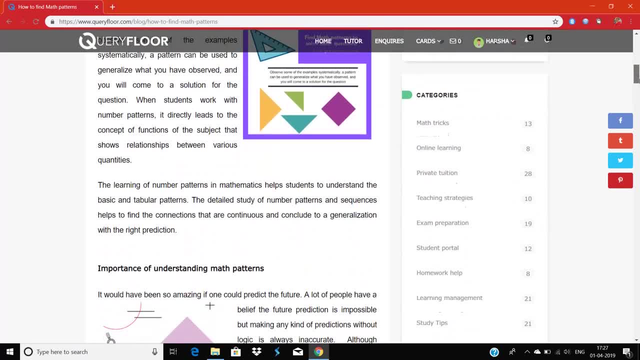 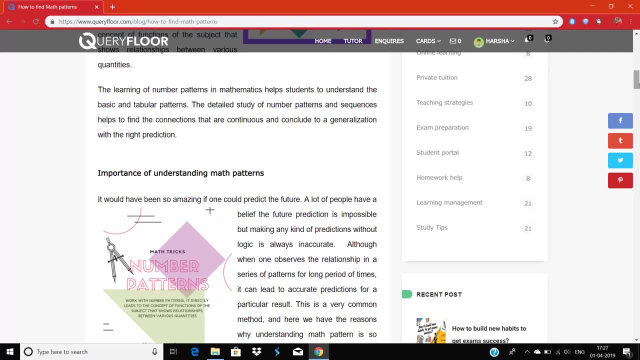 that show relationships between various quantities. The learning of number patterns in mathematics helps students to understand the basic and tabular patterns. the detailed study of the following patterns and sequences help find connections that are continuous and conclude to generalization with the right prediction. The importance of understanding these math 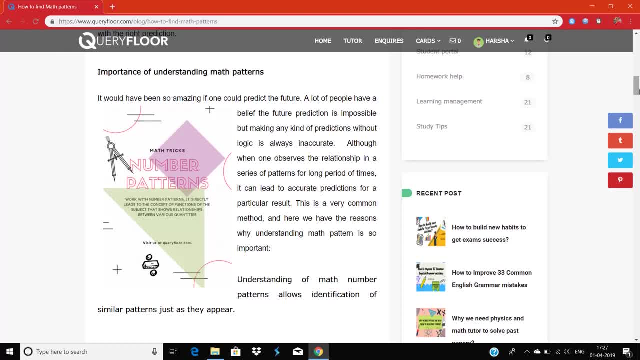 patterns. A lot of people have a belief that the future prediction is impossible, but making any kind of predictions without logic is always inaccurate, Although when one observes a relationship in a series of patterns for a long period of time, it can lead to accurate predictions. 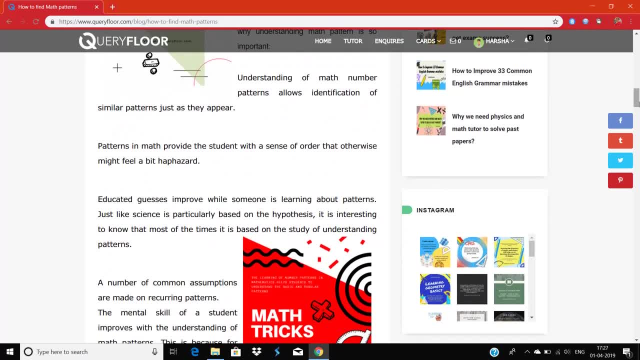 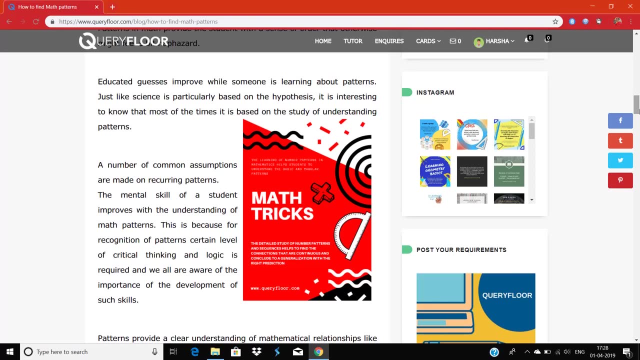 for a particular result. Understanding the math number patterns allows identification of similar patterns just as they appear. Educated guesses improve while someone is learning about patterns. Just like science is particularly based on hypothesis, it is interesting to know that most of the times it is based on the study of understanding patterns. 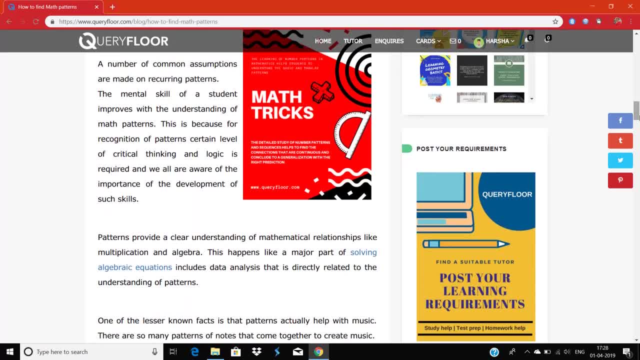 A number of common assumptions are made. The mental skill of a student improves with the understanding of math patterns and predictions. The recognition of patterns to a certain level also improves the critical thinking and logic building. We are all aware of the importance of the development of such skills. 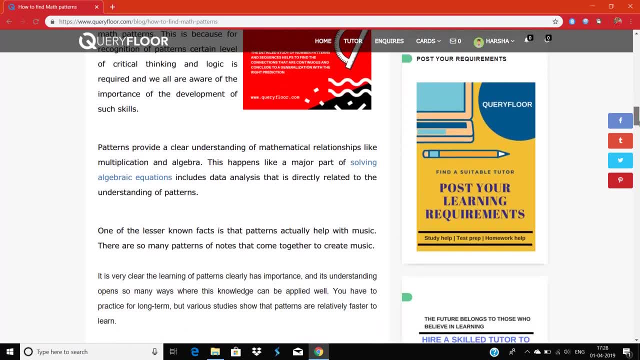 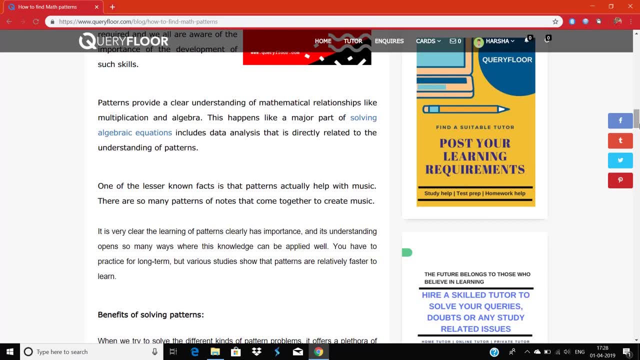 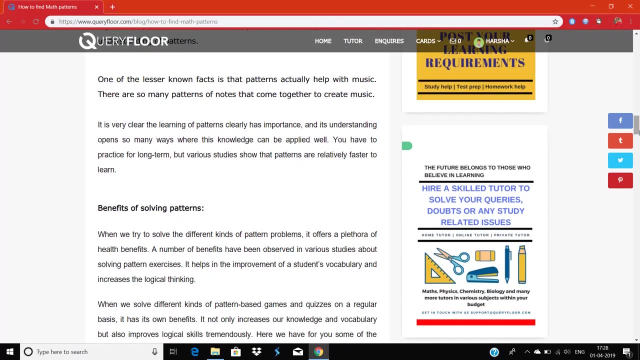 Patterns provide a clear understanding of mathematical relationships. This happens to be a major part of solving algebraic equations, including data analysis that is directly related to understanding of patterns. Also, data analytics is one of the best career options that one can pursue later in future. One of the lesser known facts is that patterns actually help. 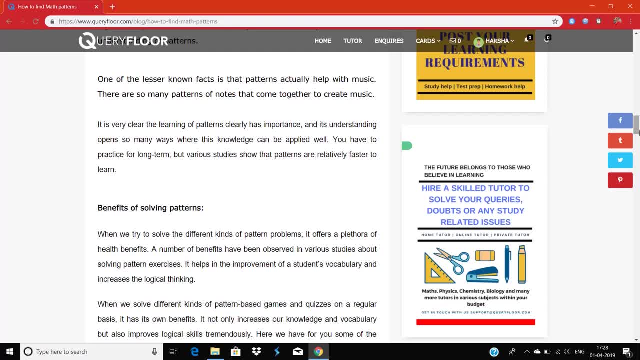 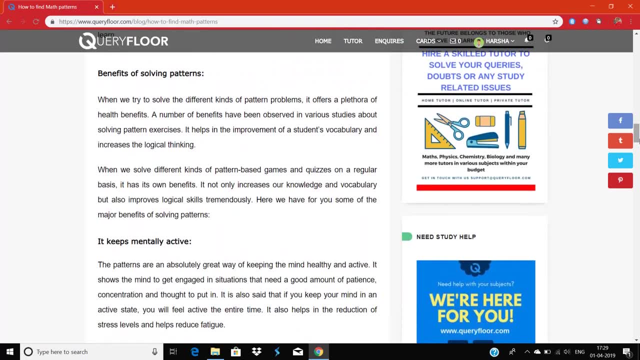 with music. There are so many patterns of notes that come together to create music. It is very clear the learning of patterns clearly has importance. The Benefits of Solving Patterns: When we solve different types of pattern-based games, quizzes on a regular basis. it enhances our memory. It has its own benefits. It also 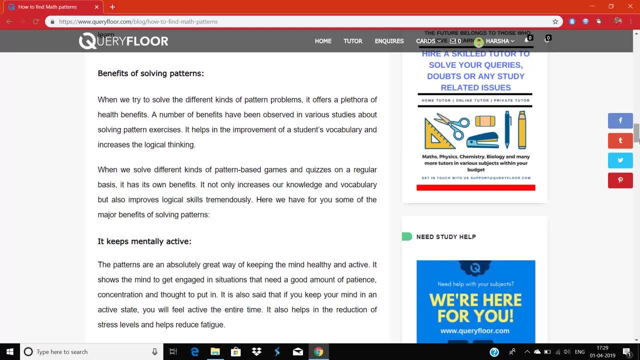 helps you think better solve problems easily. It does not increase our knowledge and vocabulary, but it mostly improves our memory. It also helps you think better solve problems easily. It does not increase our knowledge and vocabulary, but it mostly improves our memory. It also 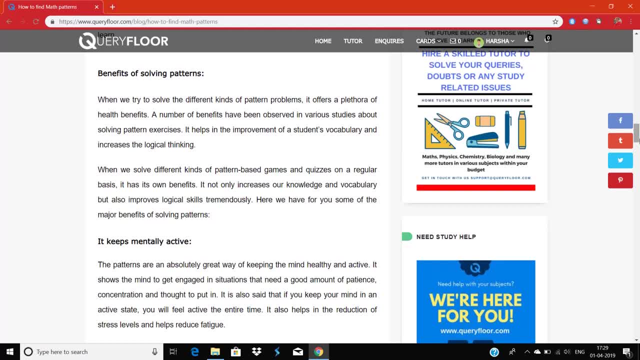 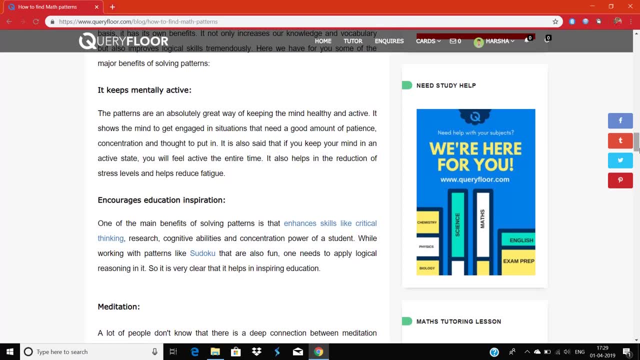 increases our logical skills. So here are some tips to keep you mentally active. Firstly, to learn patterns. it keeps you mentally active. The patterns are an absolutely great way of keeping the mind healthy and active. It shows that the mind is working in the right 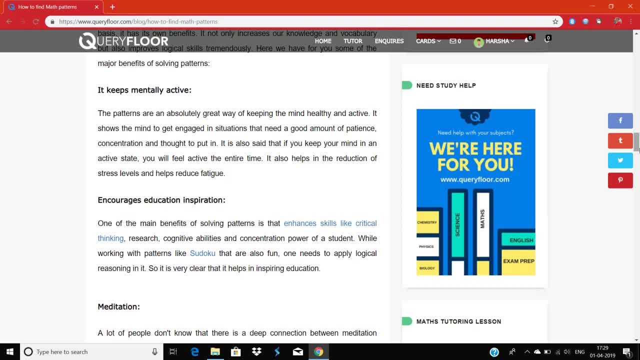 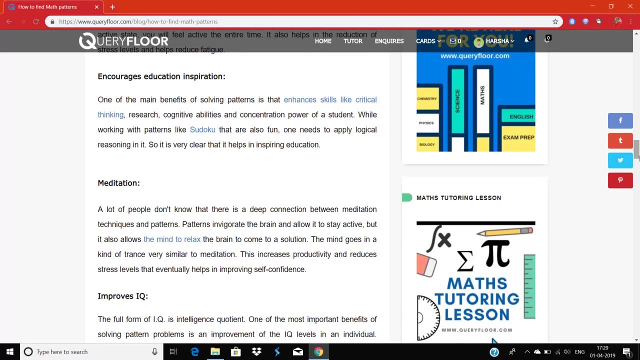 direction. It also tells you that the mind requires the right amount of concentration and thought to be put in. So it is said that if you keep your mind in a certain active state, you will feel active the entire time. It also encourages education inspiration. One of the major benefits is that it enhances 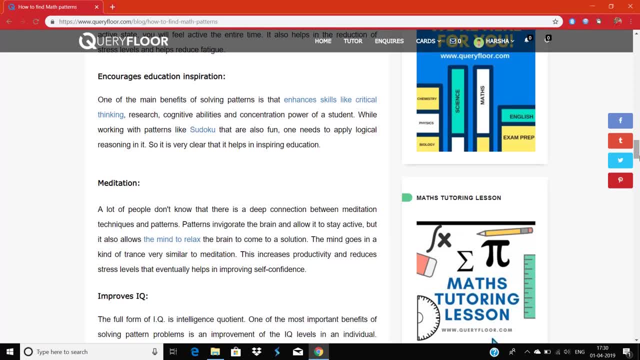 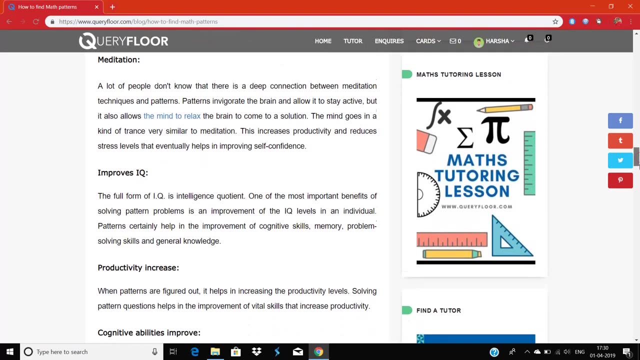 skills like critical thinking, research, cognitive abilities and concentration power of a student, While working with patterns like Sudoku that are also fun. one needs to apply logical reasoning, So it not only helps you increase critical thinking, but it also is fun Meditation. 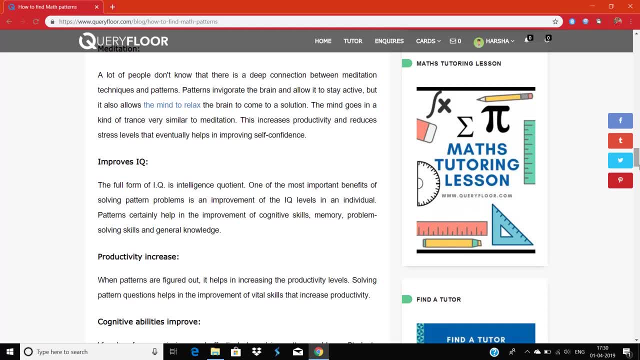 A lot of people don't know that there is a deep connection between patterns and meditation Patterns and Meditation. A lot of people don't know that there is a deep connection between patterns and meditation. Patterns invigorate the brain and allow it to stay active, But it also allows the mind 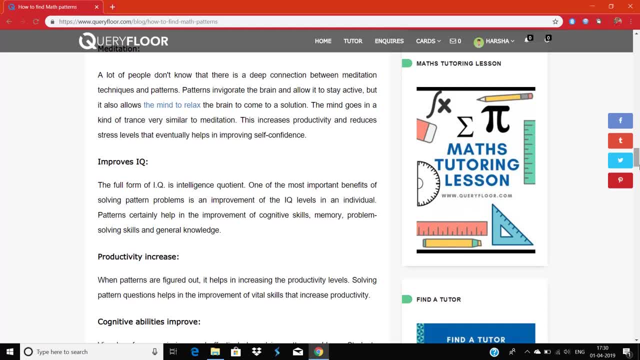 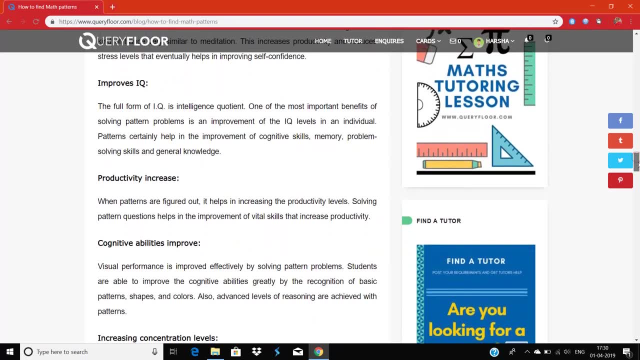 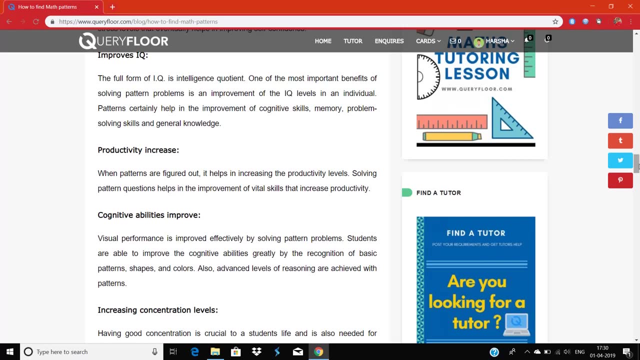 to relax. As the mind gets active, it also relaxes, So it increases productivity and reduces stress levels. It improves your IQ. One of the most important benefits of solving patterns is that your improvement of IQ levels of an individual Pattern recognition, solving, improvement of cognitive skills, memory. It. 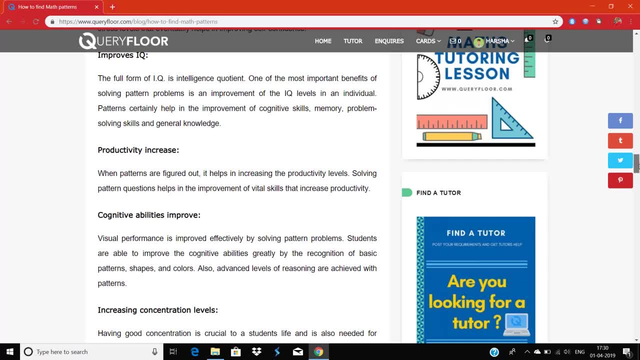 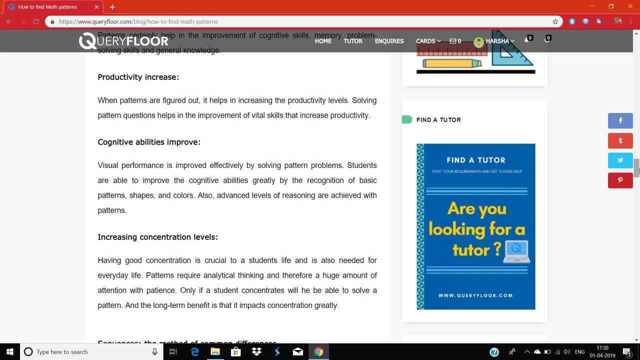 increases your problem solving skills and general knowledge. It also increases your productivity in anything that you are doing. Whenever you are doing some problem, you are at it, So it obviously increases your productivity as an individual. Solving pattern problems helps in the improvement of vital skills. 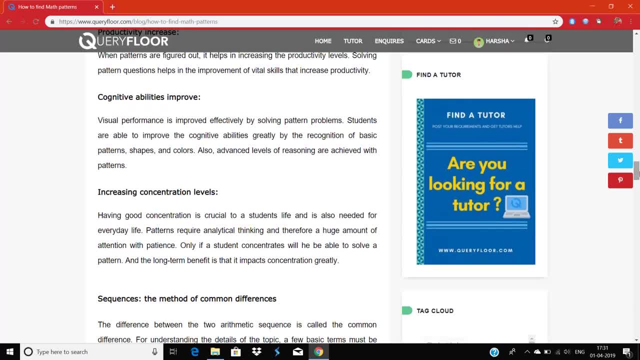 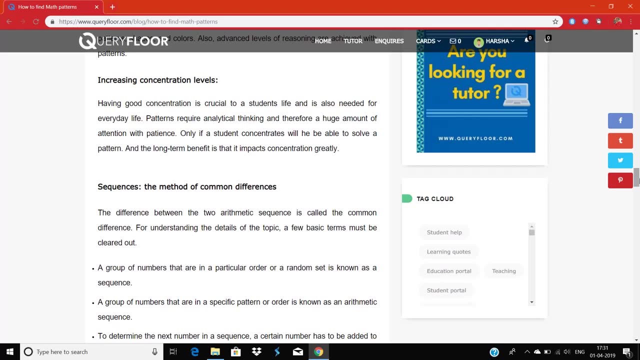 Cognitive abilities. improve. Visual performances improve. Students are able to improve their cognitive abilities greatly by recognition of basic patterns, shapes, colors, Increasing concentration, Increasing concentration levels. Patterns require tremendous analytic thinking and huge amounts of concentration and focus. If a student cannot concentrate, he will not be able to solve a certain pattern. 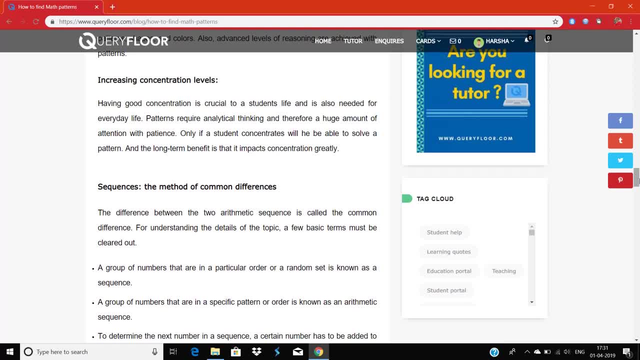 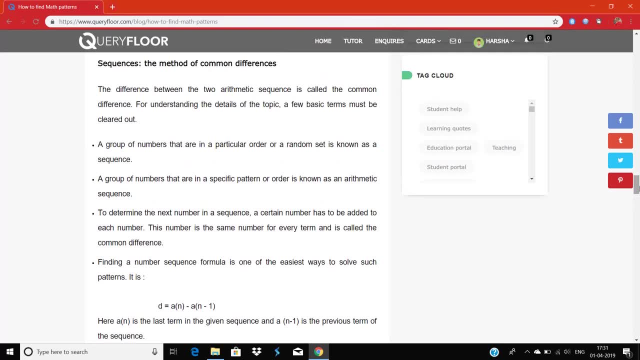 Therefore, the long term benefit is that it impacts concentration greatly. The sequence, the method of common differences: The difference between two arithmetic sequences is called the common difference. It is known as AP series. A group of numbers that are in a particular order or a random set is known as a sequence. 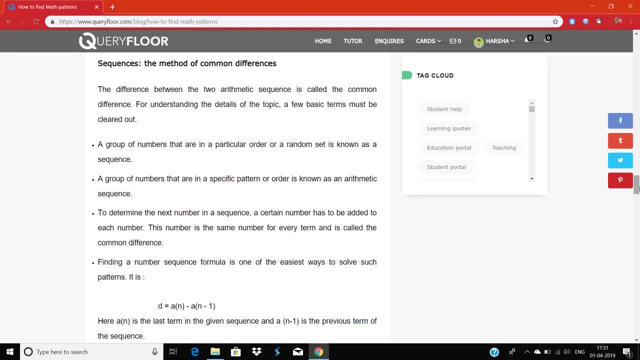 A group of numbers that are in a specific pattern or in order is known as an arithmetic sequence. To determine the number of numbers or what the next number will be in a sequence, a certain number has to be attained or added to each number. This number is the same number for: 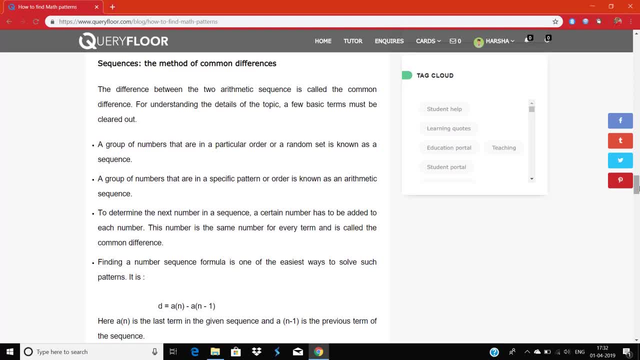 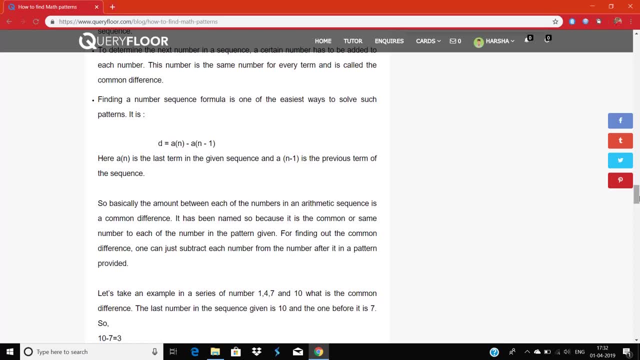 every term and it is called the common difference. Therefore, this is the formula for finding the sequential formula for forming or finding the AP series, where d equals a to the n minus a, n minus 1.. So, basically, the amount between each of the numbers is an arithmetic sequence, is a common. 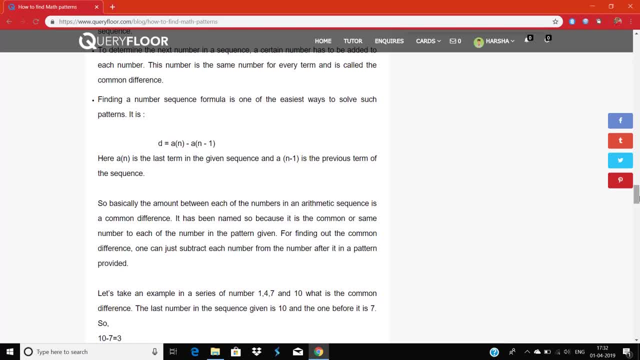 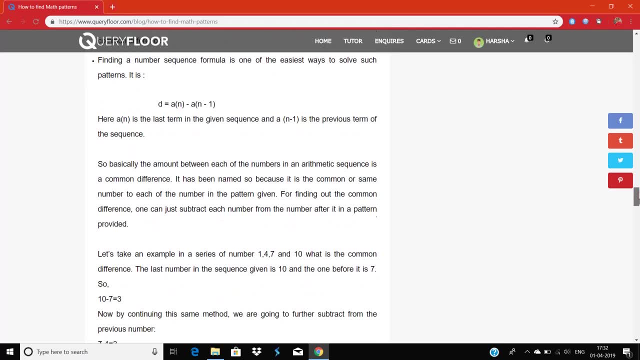 difference. It has been named so because it is the common or same number to each of the number in the pattern given. To finding out the common difference, one can just subtract each number from the number after it in a pattern. So let's take an example. 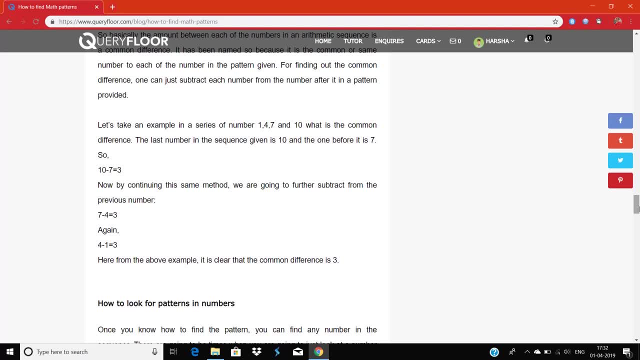 In a series of numbers: 1,, 4,, 7 and 10,. what is the common difference? The last number in the series is 10 and the one before it is 7.. So 10 minus 7 equals 3.. 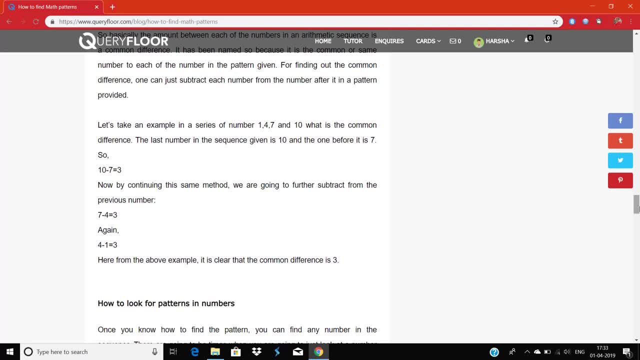 So the common difference here is 3.. Now, by continuing the same method, we are going to further subtract from the previous number: 7 minus 4 is 3.. Again, 4 minus 1 is 3.. Here, from the above example, it is clear that the common difference is 3.. 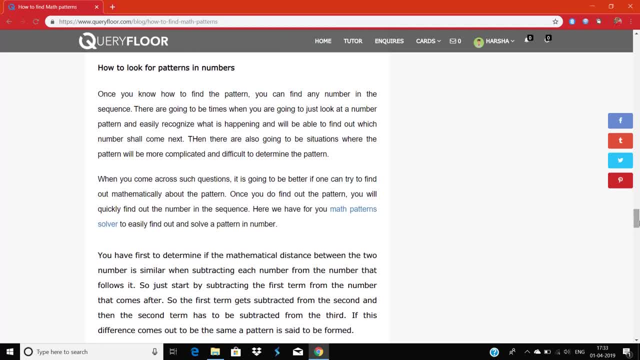 Also how to look for patterns in a sequence. Look at the numbers. Once you know how to find the pattern, you can find any number in the sequence. There are going to be times when you are going to just look at a number pattern and easily. 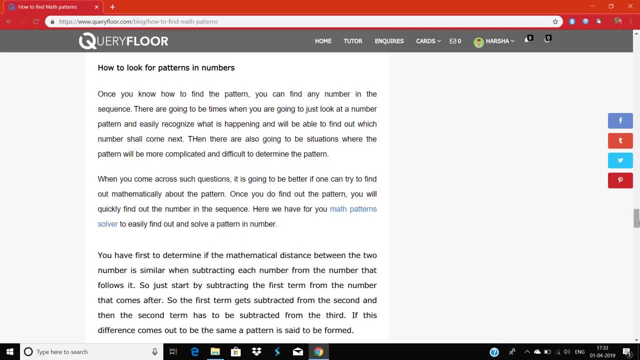 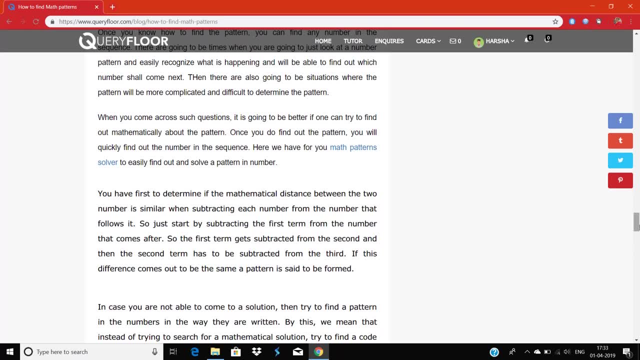 recognize what is happening and what is the next number that is going to turn up in the sequence. When you come across such questions, it is going to be easier for you to solve. You can solve it in no time. Once you find out the pattern, you will quickly find out the number in the sequence. 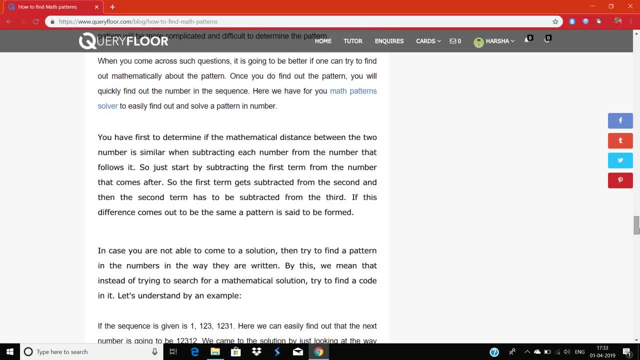 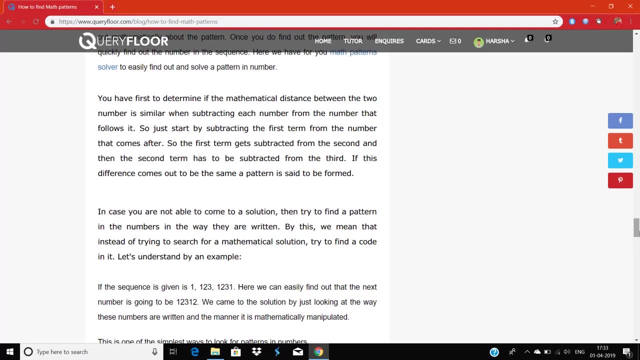 Hence it also helps you improve your math problem skills. and also to determine math patterns. You have first to determine if the mathematical distance between the two numbers is similar or not. So just by subtracting you can do that. So just start by subtracting the first term from the number that comes after it. 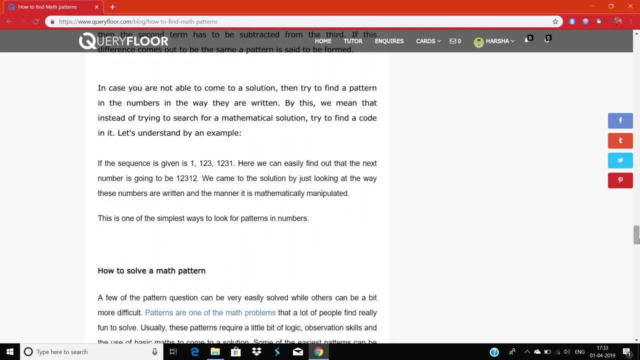 In case you are not being able to solve or come to a solution, then try to find a pattern in the numbers, in the way that they are written. By this we mean that, instead of trying to search for a mathematical solution, try to. 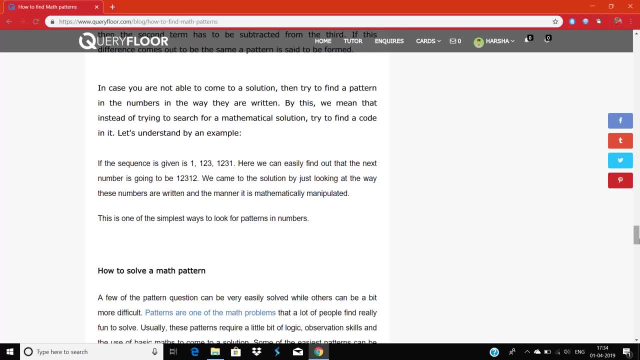 find a code in it, For example, 1, 1, 2, 3, 1, 2,, 3, 1.. Here we can easily find out that the next number is going to be 1.. 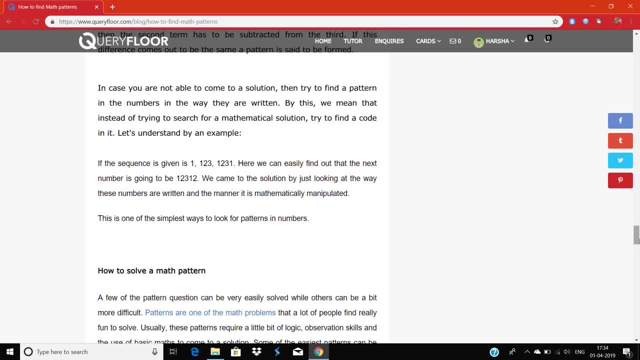 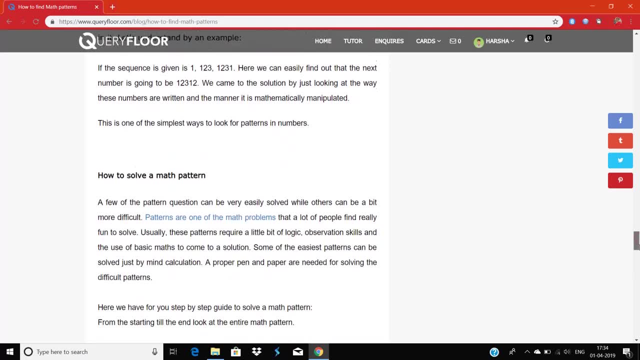 2, 3, 1, 2.. We came to the solution by just looking at the way these numbers are written, So this is one of the simplest way to look for patterns in numbers. How to solve a math pattern problem. 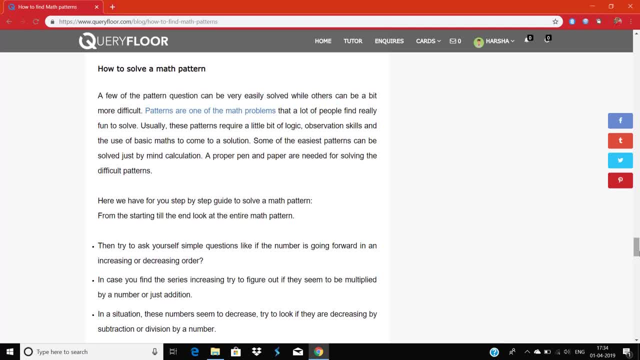 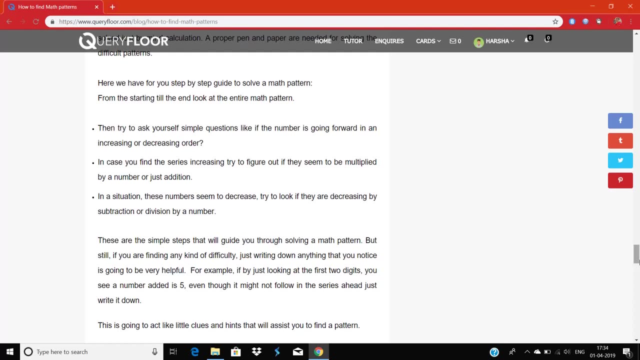 Patterns are one of the most math problems that are very difficult to solve. Usually these patterns require a lot of logic, observation skills and use of basic math. to come to a solution Here we have to do a step by step. Firstly, you try to ask yourself simple questions, like if the number is going forward in an 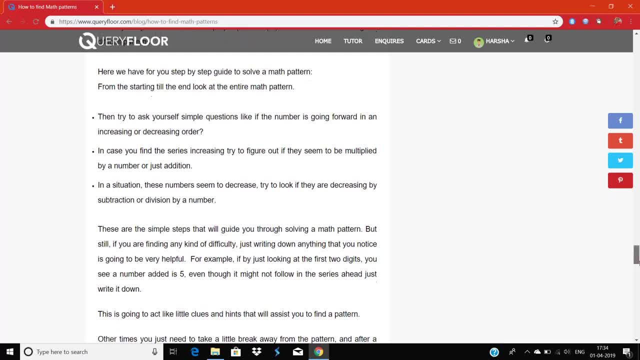 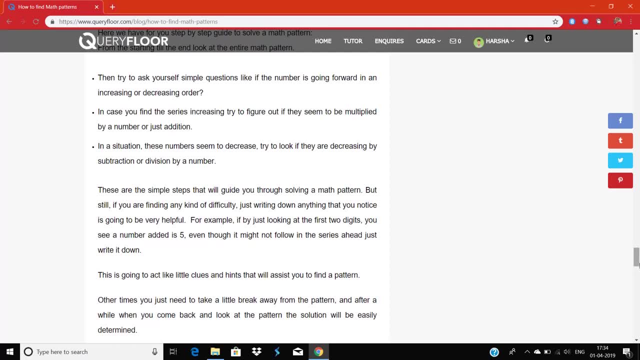 increasing or decreasing order. In case you find the series increasing, try to figure out if they seem to be multiplied by a certain number or being added to a certain number In a situation. these numbers seem to decrease, try to look if they are decreasing by a certain. 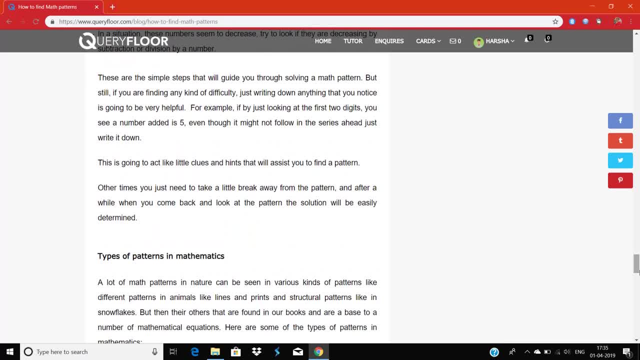 number by subtraction or by division. These are the simplest steps to follow. If you are finding any kind of difficulty, just writing down anything that you notice is going to be helpful. For example, if by just looking at the first two digits you see a number added is 5 even. 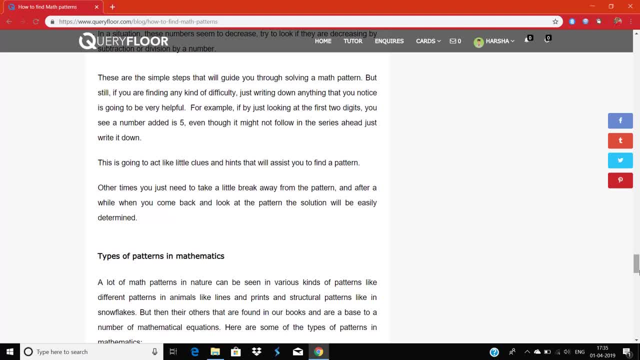 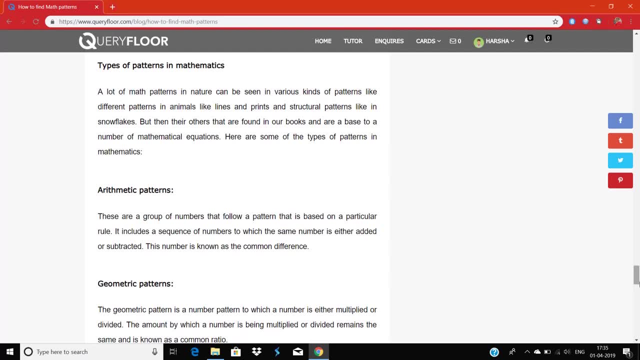 though it might not follow in the series ahead, just write it down. Type of patterns in mathematics There are a number of patterns like difficult patterns, like lines, frames, structural patterns like snowflakes, but then there are others that are found in our books and are a base. 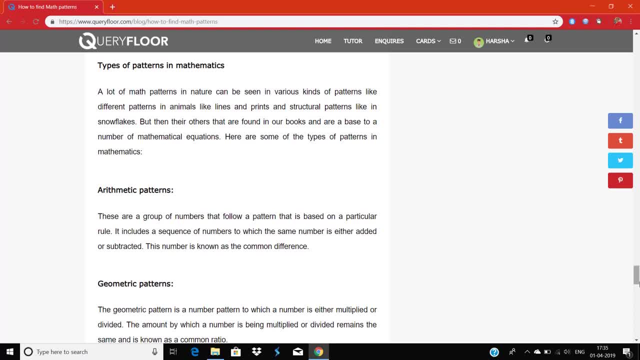 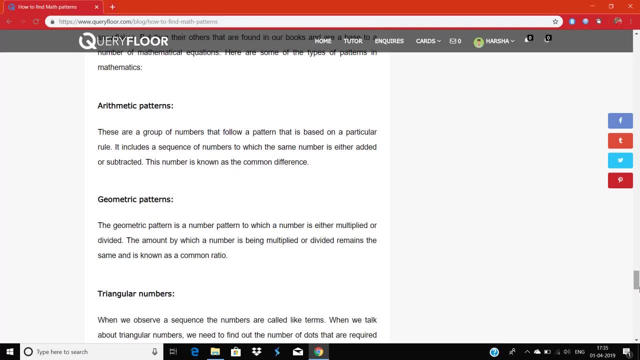 to a number of mathematical equations. They are arithmetic patterns, like we discussed, and AP series. These are a group of numbers that follow a pattern that is based on a particular rule. It includes a sequence of numbers to which the same number is either added or subtracted.